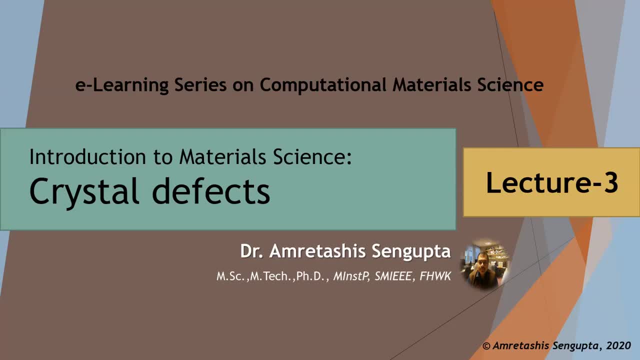 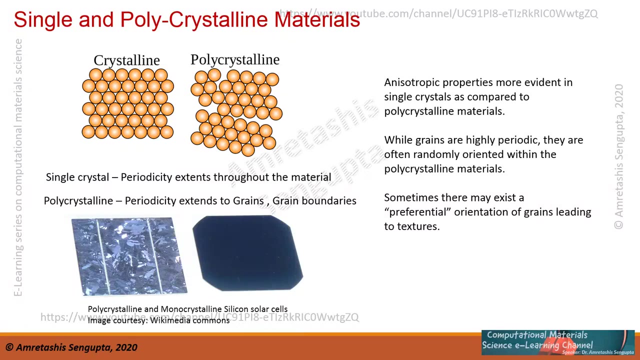 Namaskar, hello friends and welcome to another edition of this lecture series on material science, And today we will talk about crystal defects. So we know that there are these single and polycrystalline materials. In single crystal, the periodicity will extend throughout the entire material. 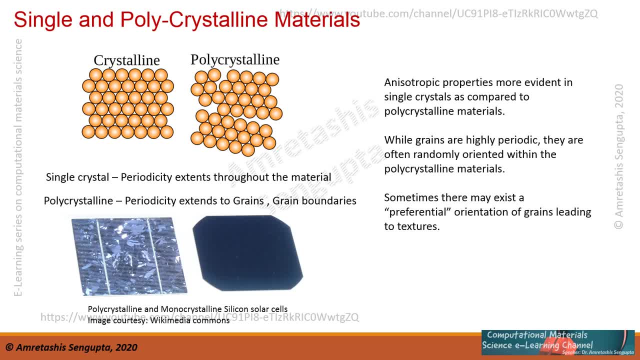 And in polycrystalline solids the periodicity extends to grains and these grains are oriented somewhat randomly with respect to one another and they touch each other at grain boundaries. So naturally in a polycrystalline material there is anisotropic properties. 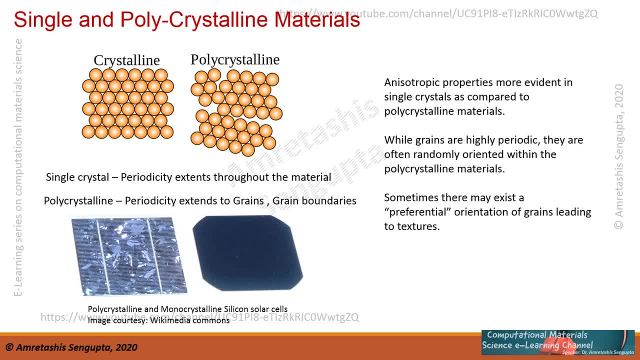 This would be somewhat less as compared to single crystals and because the more randomly the grains are oriented, the more deviation from anisotropy might be there. But sometimes there also might exist preferential orientation of grains and that gives something called texture to a material. 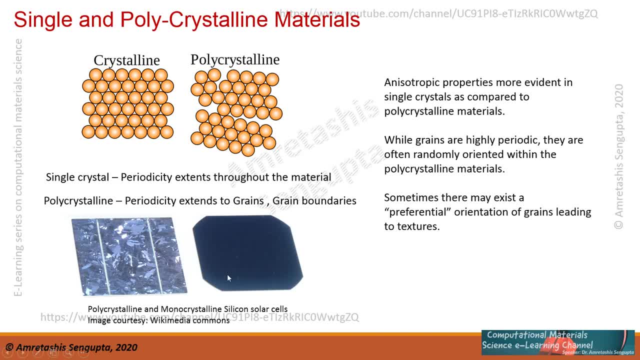 And even with the bare eye it is possible to somehow identify single and polycrystalline materials Sometimes, for example, this monocrystalline silicon solar cell and a polycrystalline silicon solar cell. So this one is a polycrystalline one and we can see there is this very nice pattern, this structure. 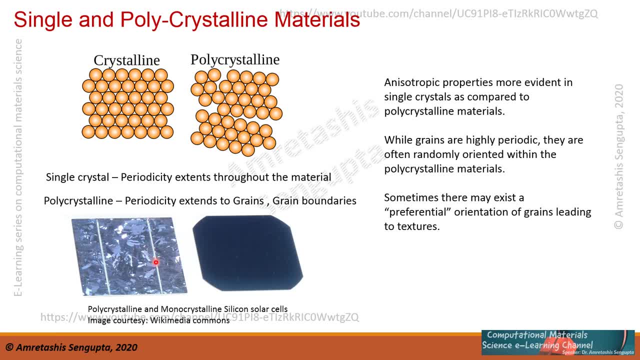 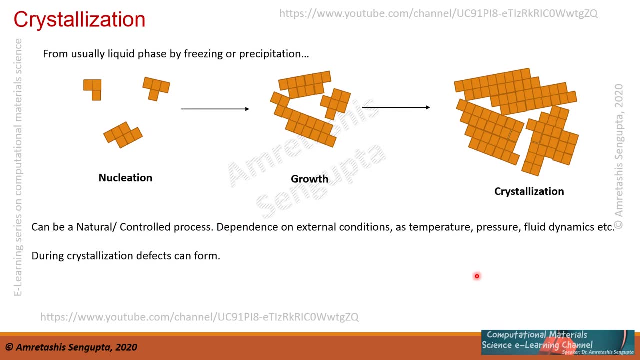 Different crystallographic planes are exposed in this case and they are reflecting light differently, So you have this kind of a texture as compared to this one. Now, crystallization is the process in which, from a liquid phase, usually, a crystal forms by freezing or precipitation, in some cases from a gaseous phase. 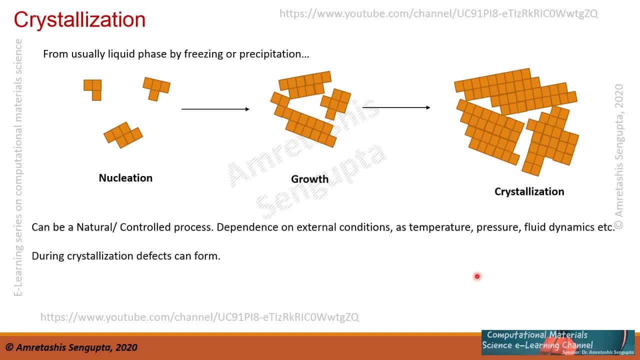 There might be some chemical reactions, and then you have some kind of deposition, like in the CVD process, And let us just limit ourselves right now to the formation of crystal from liquid phase. And there you have this nucleation where nucleation centers appear very highly: periodic regions. 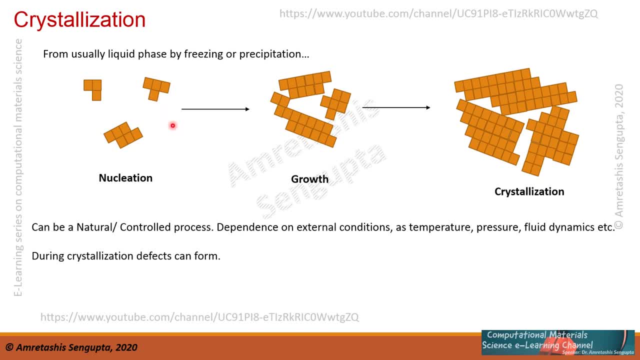 And from these nucleation centers the crystals start to grow, and this here is a polycrystalline solid. So these nucleation centers grow and come together to form the polycrystal. Depending upon the condition, it is also possible to form single crystals in this way. 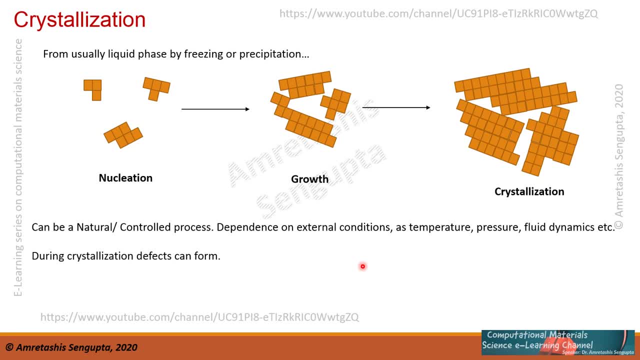 So the process might be natural or might be a controlled process. For example, the growth of silicon, The growth of silicon wafers when silicon highly ordered and oriented silicon crystal ingots are grown from the melt. So that is a controlled process. 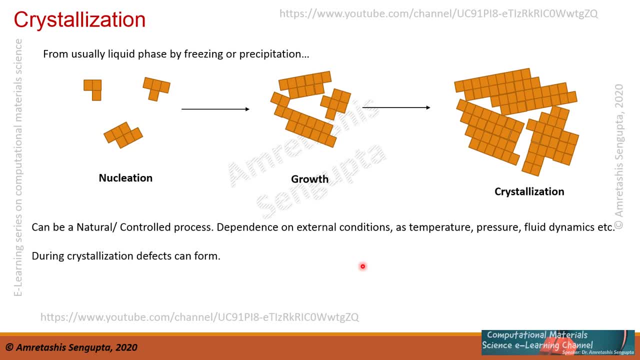 And whether in natural or in controlled process, there is always still some amount of fluctuations might be there. And so lot of external growth, So lot of external conditions determine how the crystal growth is taking place. So temperature, obviously, pressure, and if it is forming from a liquid phase, how the fluid dynamics plays out. 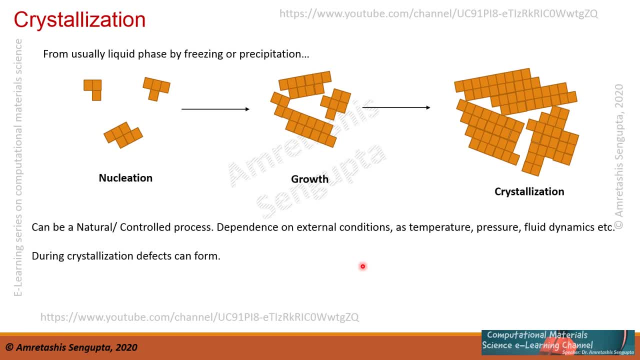 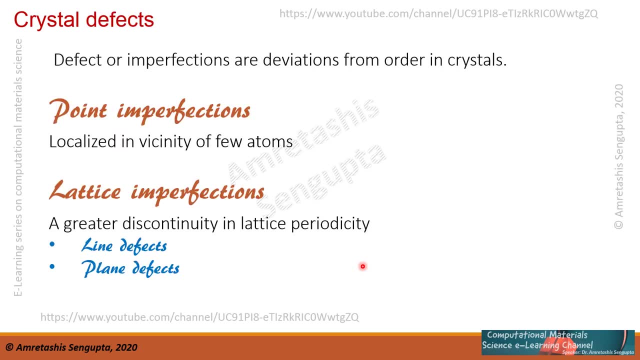 All these things will impact the crystallization And due to that, defects can form. And talking about crystal defects, Basically they are deviations or imperfections from a perfect order in crystals, So they can be classified into point: imperfections which are localized in vicinity of a few atoms. 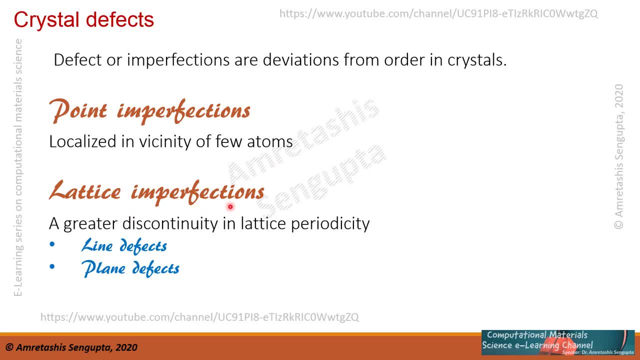 And maybe lattice imperfections, where the greater discontinuity is there in lattice periodicity, So it is on a larger, much larger scale- Affects the lattice much more. And among these lattice imperfections you can consider these line defects and plane defects. 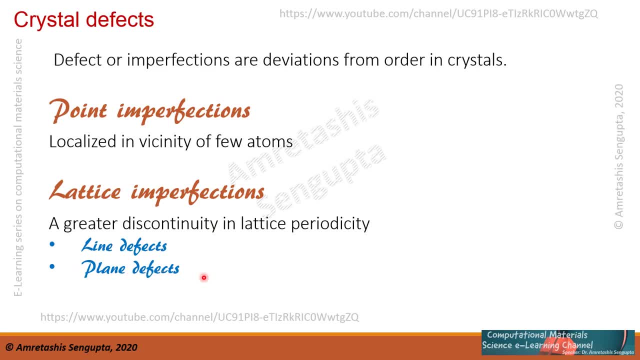 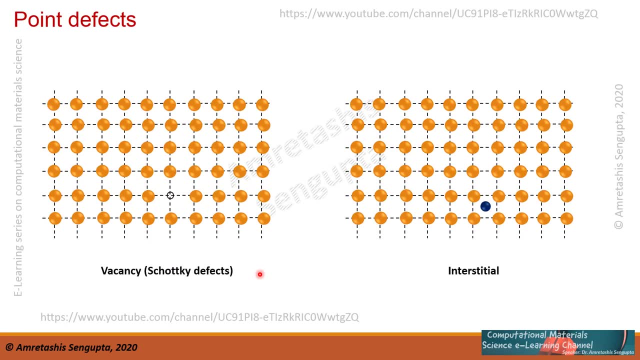 So line defect is along a line and plane defect is along a plane. Now let us talk initially about the point defects. So then there are this different type of defects we are going to show And very simple two-dimensional example. I am taking a square two-dimensional. 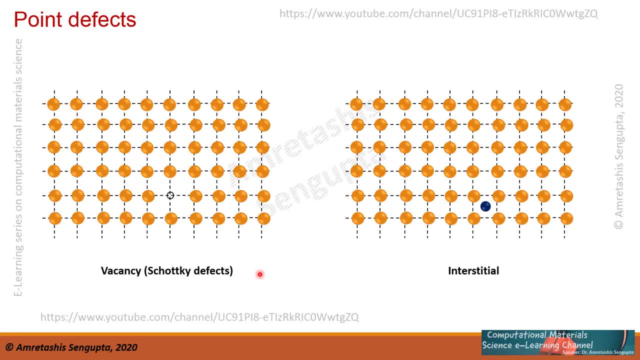 I am taking a square 2D lattice. In a real case we have a much complex 3D diagram, But just to simplify we present it this way And you can see if an atom is missing from its designated position. So that is called a vacancy. 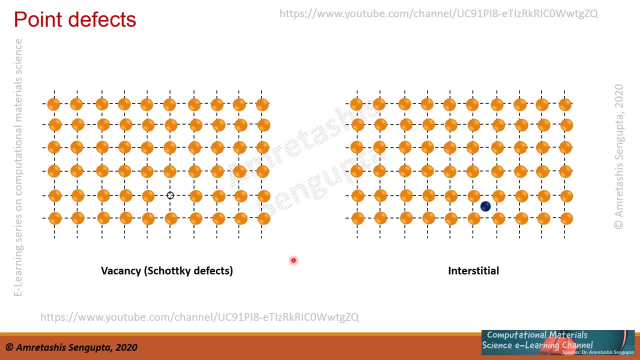 And also sometimes it is called a Schottky defect. Maybe one, Maybe more atoms might be missing. So this kind of point defects are known as Schottky defects or vacancies. Then there can be interstitials, So these vacant spaces in between the occupied positions. these are called interstitials. 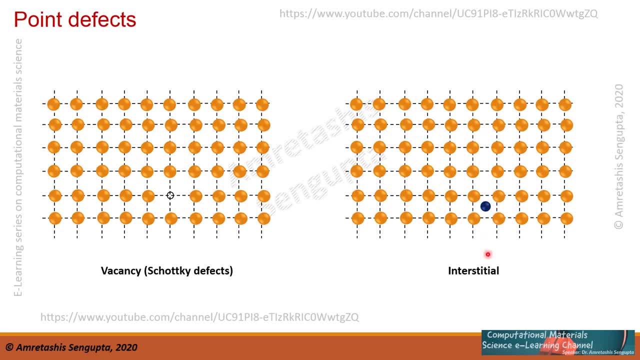 And in this interstitial there might be foreign atom that can some impurity, or foreign atom that can come in. Sometimes also it is an extra atom of the same material. So this kind of defect is known as the interstitial, because it is sitting in an interstitial space. 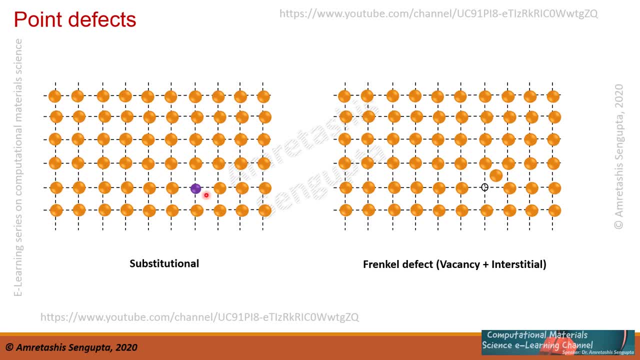 Then there can be substitutional impurity, So one of the atoms of the original lattice is taken out and replaced by some other foreign or impurity atom. It might be due to some processing Or might be intentional, as in the case of doping. 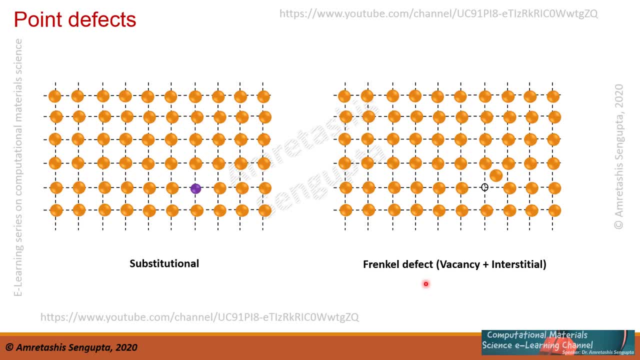 And then another very interesting point defect, the Frenkel defect, which is caused by vacancy, and an interstitial. So in some cases the atom might be dislossed from its original position And it can go into the interstitial space. 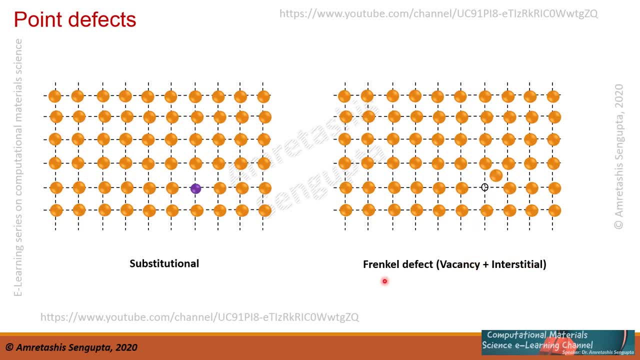 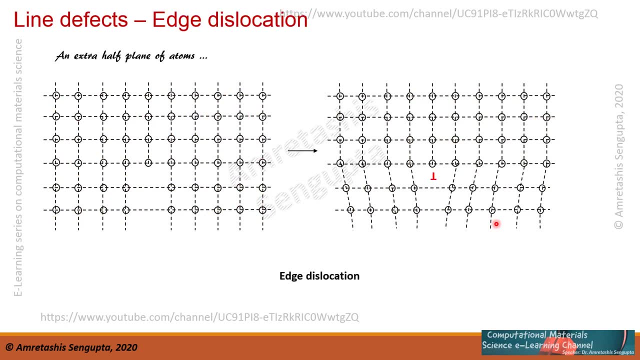 And this interstitial and the vacancy together it is called the Frenkel defect. We now come to line defects And these defects are happening along a line. So in case there is again with this 2D lattice. I show the example. 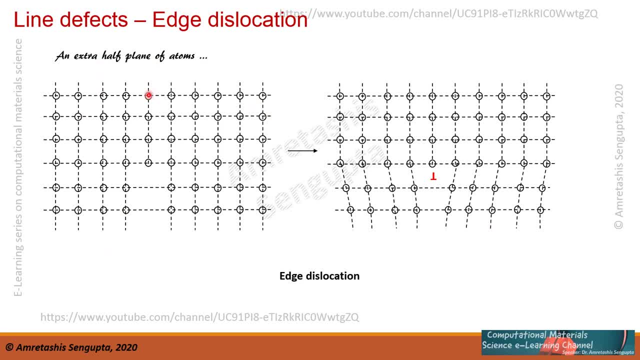 So say, for example, there is an extra half plane of atoms. So this is a 2D picture. You can imagine A set of planes, These planes to continue, say, for example, going into the paper, or rather the slide. 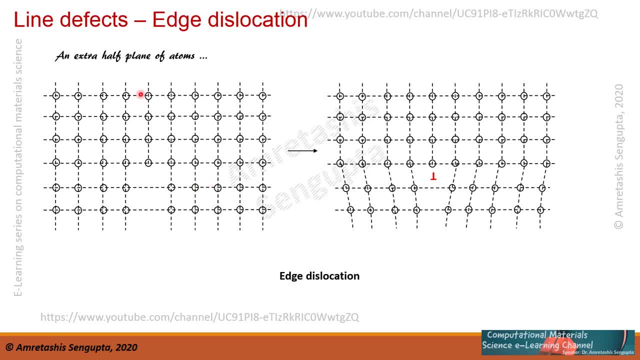 So we can think like that, And I am just showing the 2D picture. So from that, this particular plane, you see, is different from all the others Because it is only up to this halfway mark, It is not extending throughout the whole crystal. 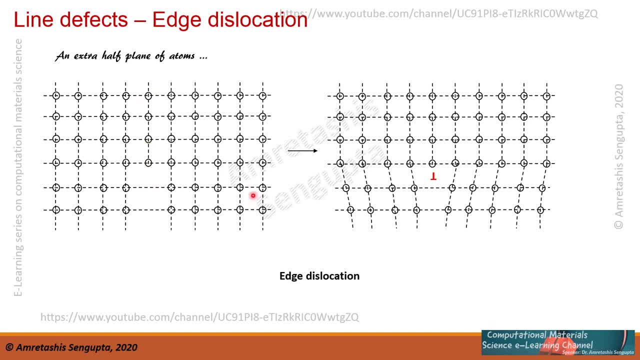 And this kind of a defect will go on to stabilize in something like this Because this half plane is missing, or you can also think of it as an extra half plane being introduced, Whichever way you look at it. So this kind of a dislocation is known as an edge dislocation. 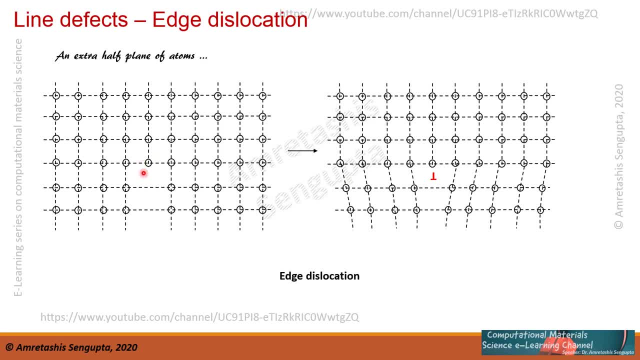 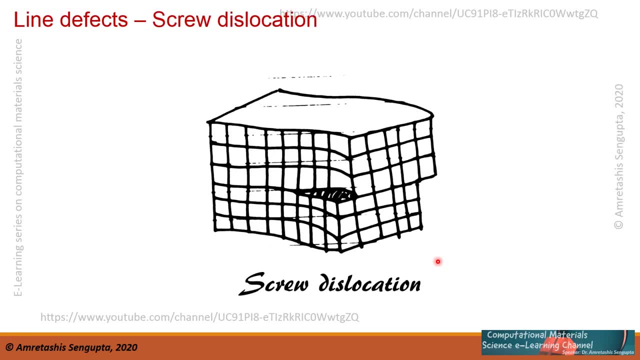 Because it takes place around the edge of this sort of a plane. And then there is another type of line defect: The screw dislocation. So here you see, the diagram is a little bit rough, But still you can understand that there is some sort of a shearing kind of a force at play. 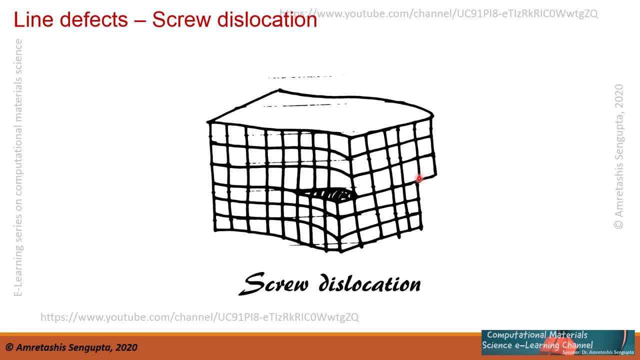 And that sort of distorts the order a little bit And it has sort of pushed this region away And created this kind of a region right here. So the 2 planes are not perfectly aligned right here. So this kind of a dislocation is known as the screw dislocation. 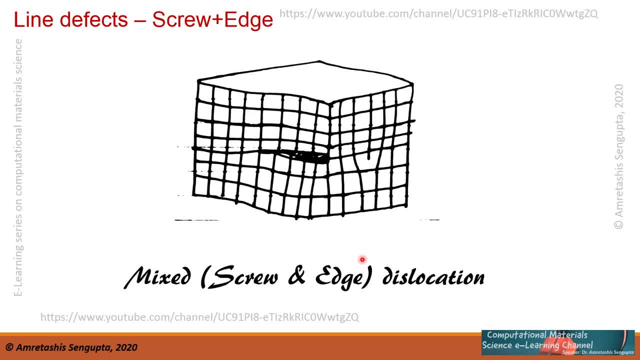 And another kind of line defect can be there where there is a mixture of screw and edge. So here we see that there is obviously a screw And also an extra half plane or a missing part of a complete plane is there And that is an edge dislocation. 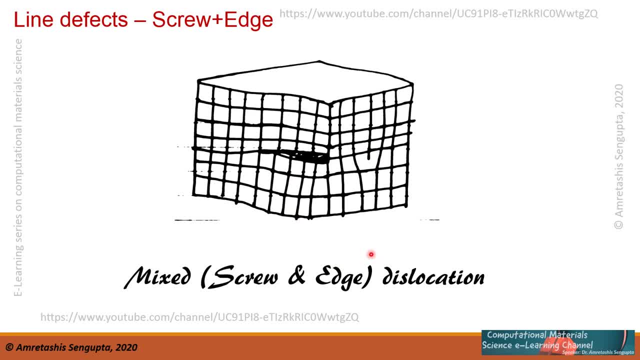 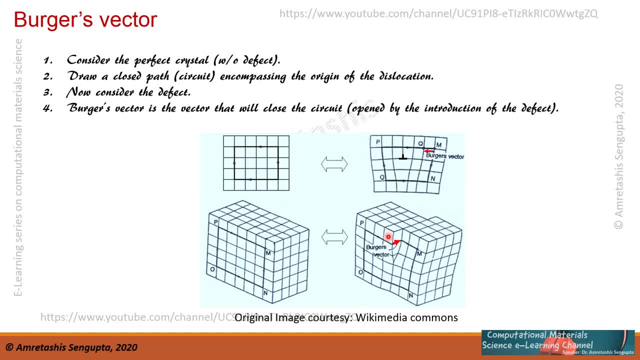 So edge and screw combine to make a mixed dislocation. And now we come to a very important point. We come to a very important geometric construction known as the Burgess vector. So this is such a vector which can be used to represent a crystal defect. 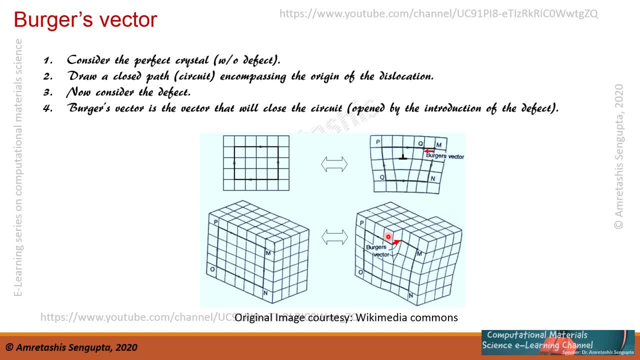 So how to construct this is: first we consider the perfect crystal that is without defect, Say, here I have taken this one. And then you draw a closed part circuit encompassing the origin of the dislocation Like this: So I know that there is a defect. 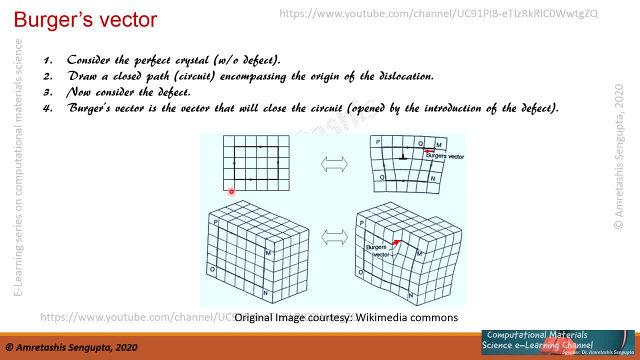 But first I draw a circuit in the perfect case, encompassing where my defect is, But I do not introduce the defect yet. And then I introduce the defect after the closed circuit I have drawn. So this is a geometrical construct in your mind. 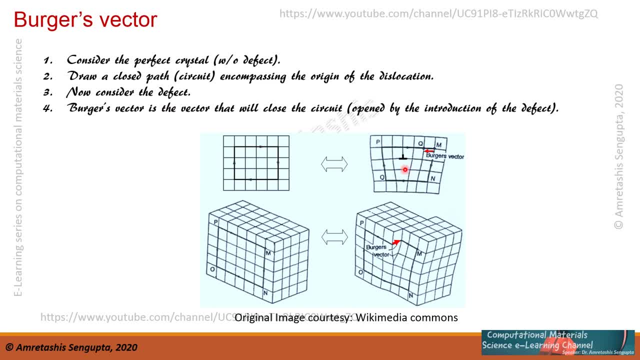 And then what happens is, once you introduce the defect, The closed circuit would become open, And the vector that will once again close that circuit is known as the Burgess vector, And that vector will in fact be utilized to represent this defect. So this is the Burgess vector in this case. 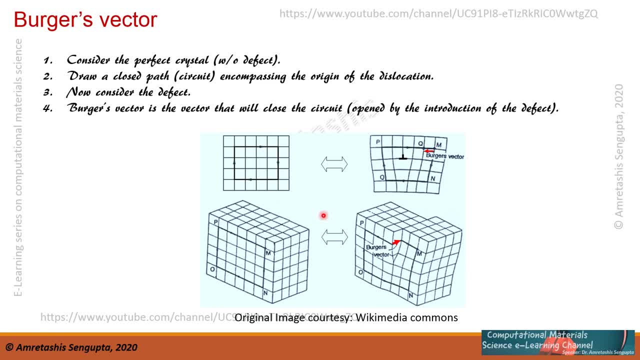 And this circuit is called Burgess circuit And also this one is for the edge dislocation. In case of screw dislocation, you can do it like this: Draw a closed circuit around this And then I know the defect is here. So I take the perfect case, draw the closed circuit. 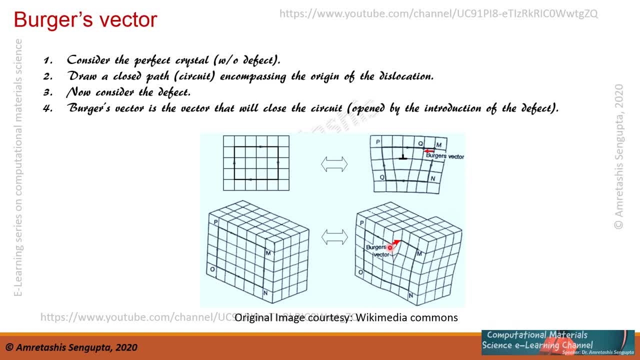 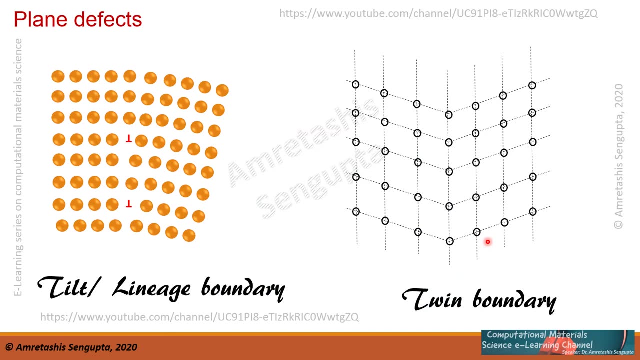 Then introduce the defect And then it becomes open, And this is the vector that now will close the path once again. So that vector is the Burgess vector, Another kind of plane defect we are talking about. So these were line defects. 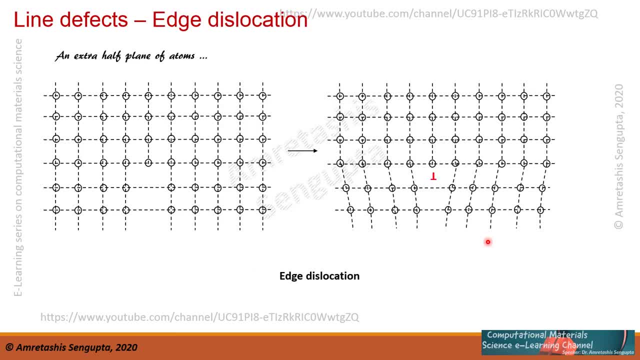 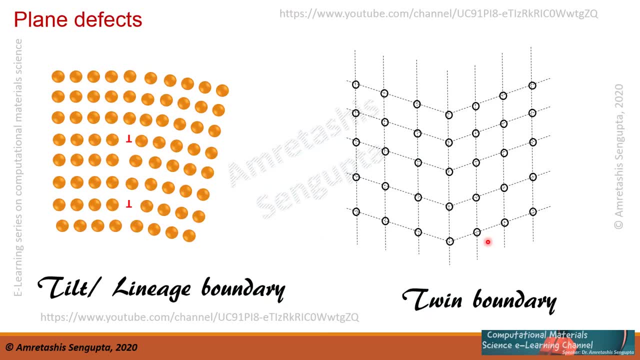 Screw dislocation, edge dislocation and these things, Because they are along a line. And then there are plane defects And there is this tilt or lineage boundary among plane defects Which is caused by multiple edge dislocations, And there is a twin boundary which looks somewhat like this: 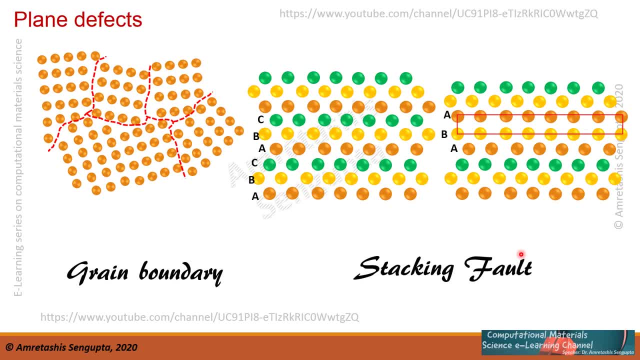 And further there are the grain boundaries. We talked about the highly oriented grain regions in a polycrystalline material. So the grains are perfectly oriented And one grain relative to another is randomly oriented. So among these grains you will see this grain boundary regions by these dashed lines. 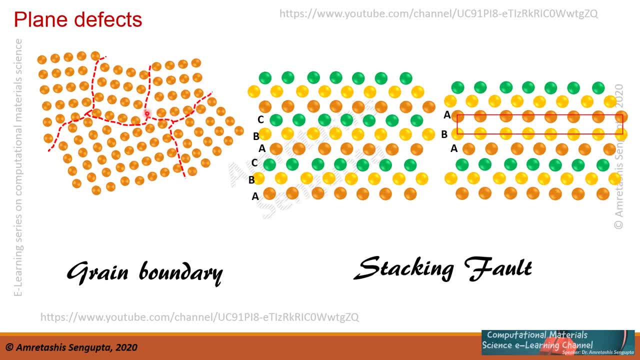 So this is a hypothetical construct And this kind of grain boundaries are very important from the perspective of chemical phenomena And etching adsorption, also electronic properties. There is scattering at grain boundaries And many other interesting things going on, And then finally there is this stacking fault. 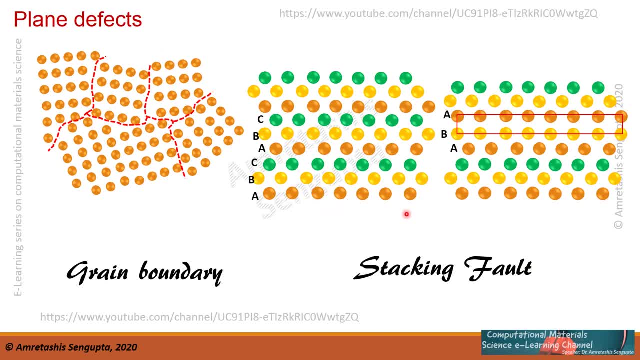 Say, you have a packed structure And it is built up with this ABC, ABC stacking. So I am just showing you the vertical direction, Not the horizontal plane, in plane direction. So this is just a side view you can imagine. So this ABC, ABC, this kind of stacking is going on here. 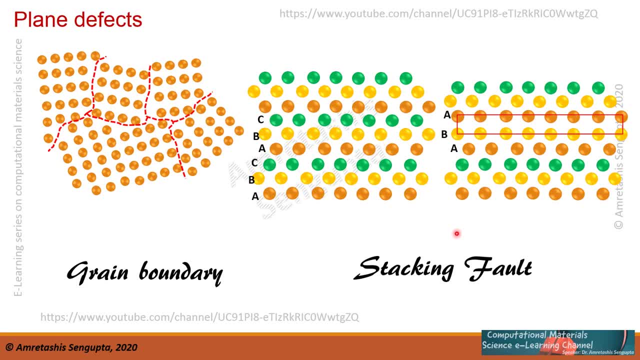 And suddenly One of the planes might be missing. And then, like here, You see, there is no C, But just again B, followed by A, And this kind of a defect is known as a stacking fault. And this can also happen in crystal and is another type of a plane defect.